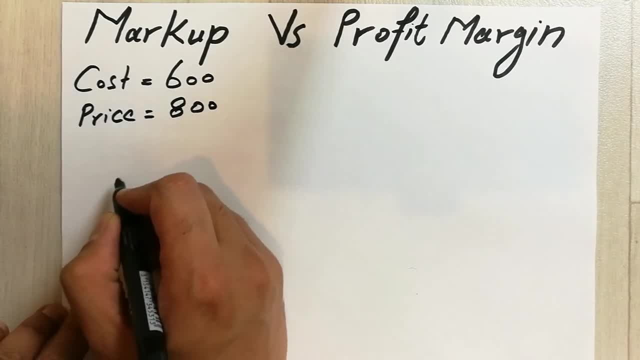 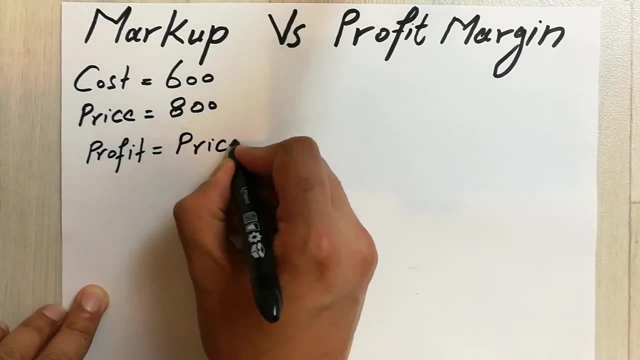 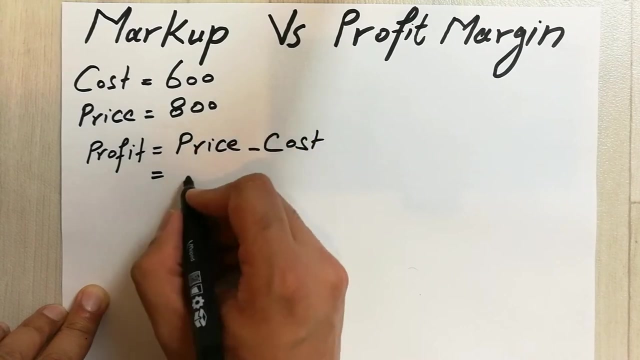 So this is the selling price. Okay, now, in the first step, we will find out the profit. Okay, so the formula to find out the profit is really simple: It's price minus cost. Okay, so now we'll put the values. Okay, the price is 800. 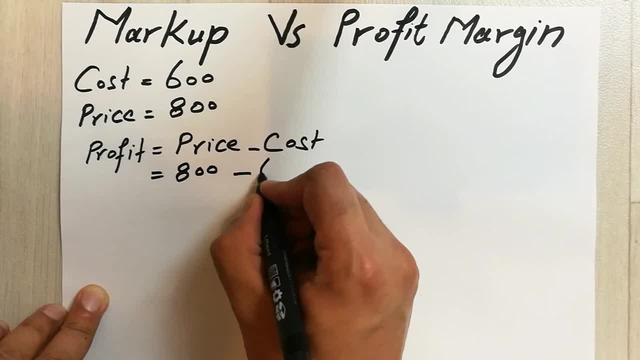 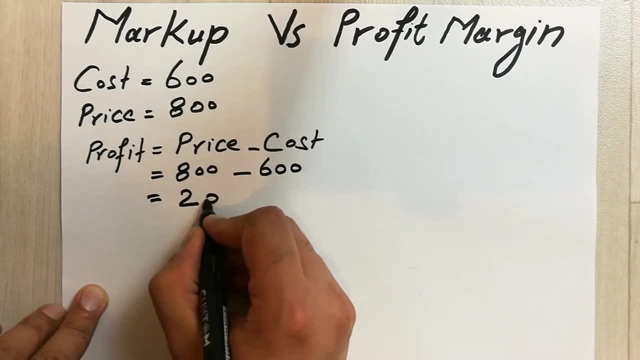 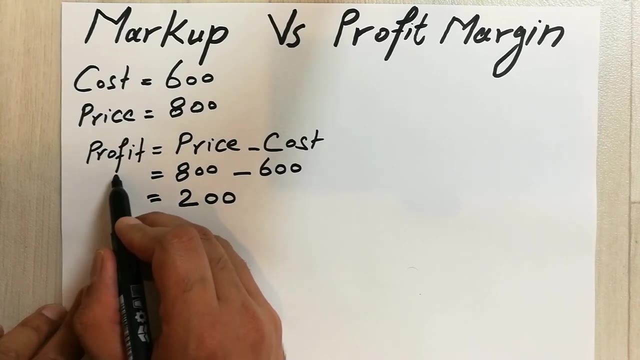 minus cost is 600.. Okay, guys, the answer will be 200.. Okay so, guys, this is our gross profit. So the profit I mentioned over here is gross profit. Okay, now, simply, what we will do. we will put the formula. 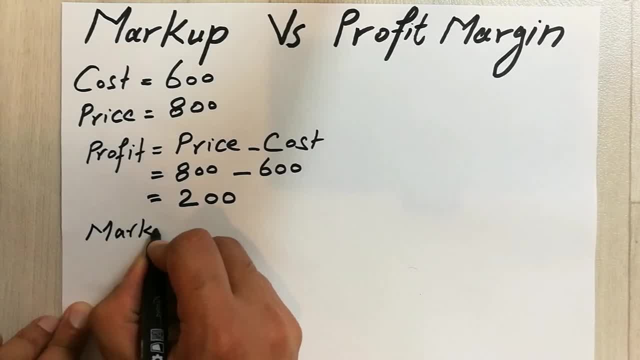 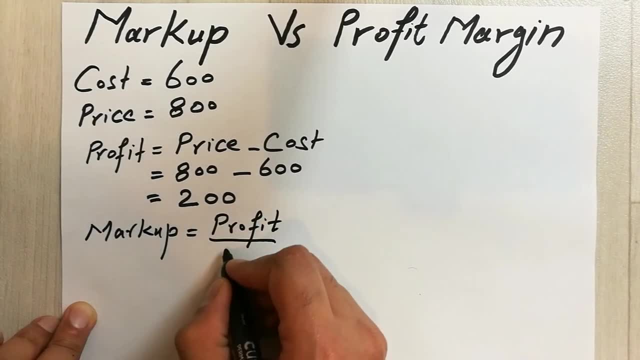 for markup. So the formula for finding out the markup is profit divided with cost. So, guys, we already find the profit. So profit here is 200.. So we'll put the value over here: 200, and our cost is here, which is 600. 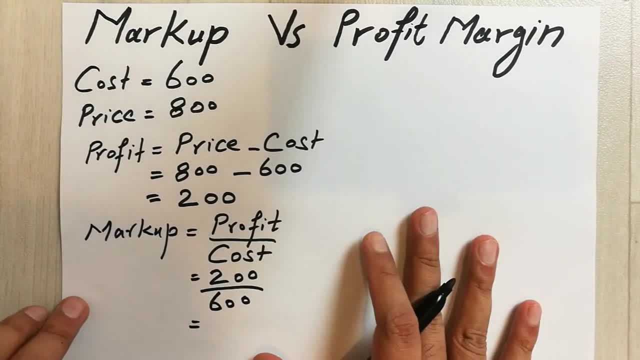 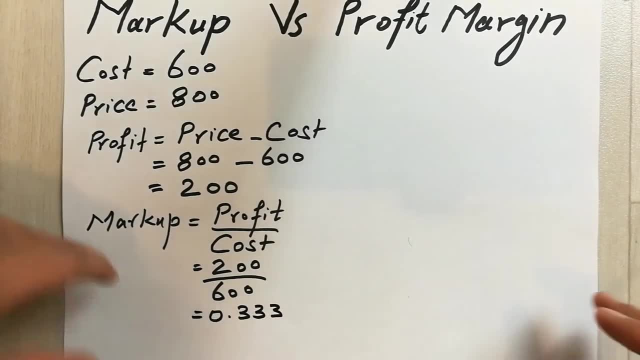 So our answer: 200 divided with 600, the answer will be 0.333.. Okay, and now to make it a percentage, we will put the value of 0.333.. What we're going to do, is we're going to do, is we multiply it with a hundred, did we? 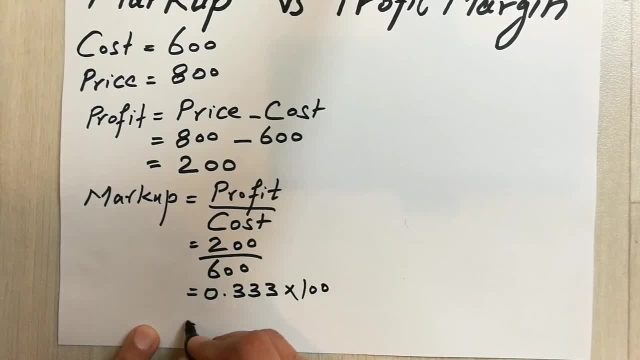 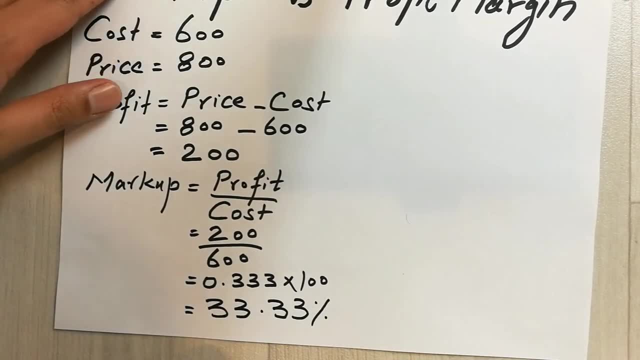 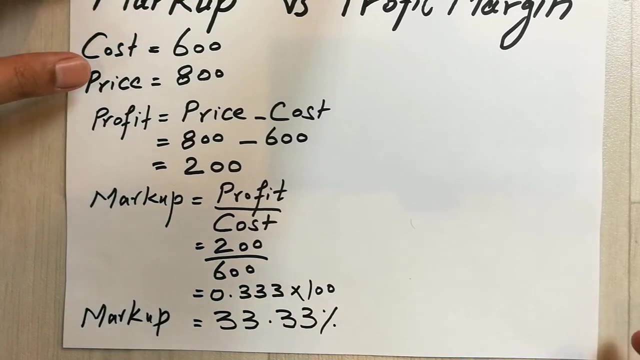 And here 100 loud. So our answer will be 33 point 33 for Percent. expensive prices are around the capital markets. So that was our markup. Okay, so in the next step we will find out the profit in March. So then we will find our profit margin. Okay, we already have the value over here족. 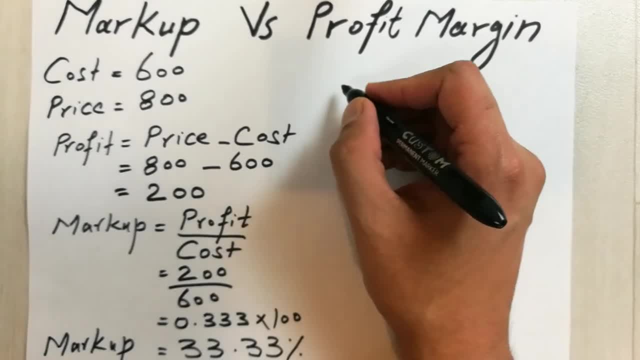 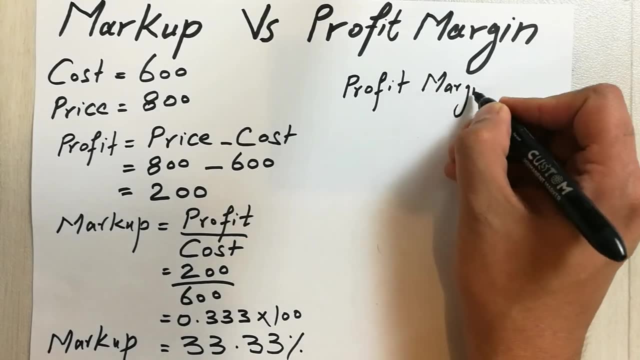 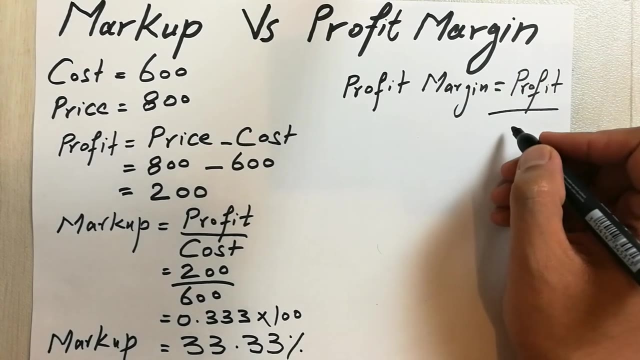 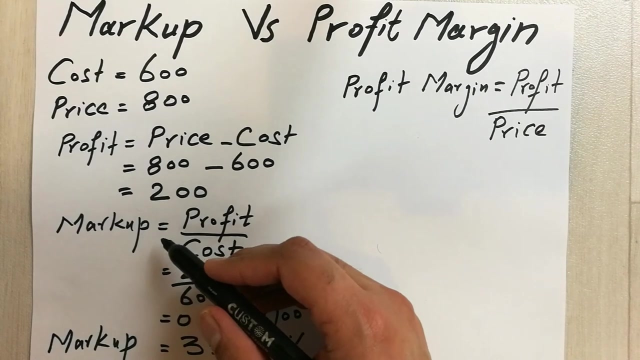 All the values over here, Zozzie values over here. so simply, we will put the formula for profit margin. okay, so the profit margin is equal to profit divided with price. so, guys, you see over here, the formula for markup is profit divided with cost. but for the profit,